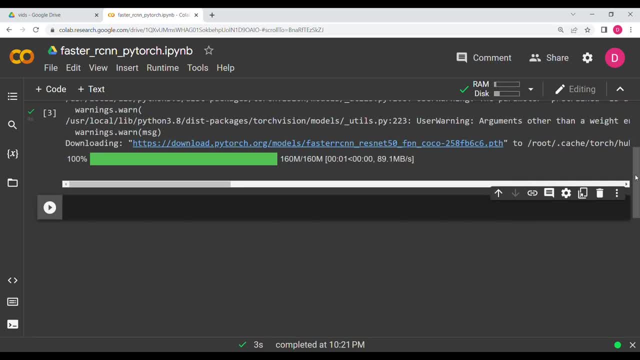 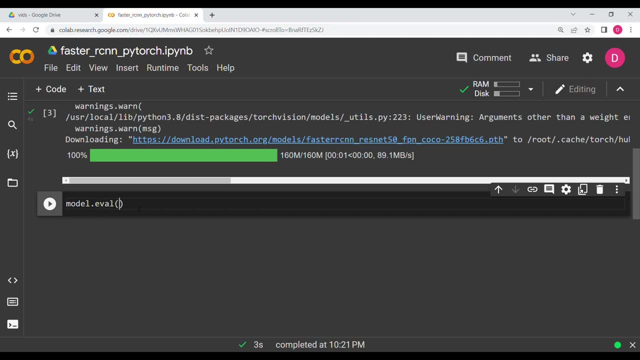 So it has, it is downloading the weights and it has downloaded the weights over here And now what we are going to do is we are going to say model dot eval. The reason, as I explained earlier, we are just going to do inference, Which means that we are not going to do any fine tuning. 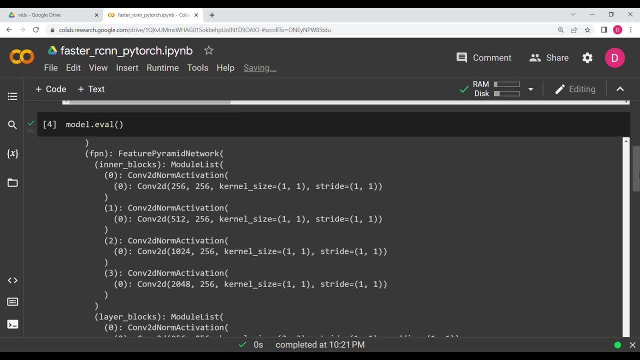 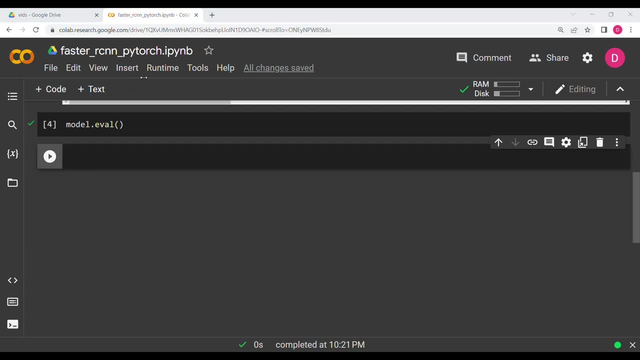 So this is the model parameter. These are the model. This is the model architecture. We will close this over here and after that. now I need to get the image, So the link for the image is already in the description below. I'll just copy and paste it over here. 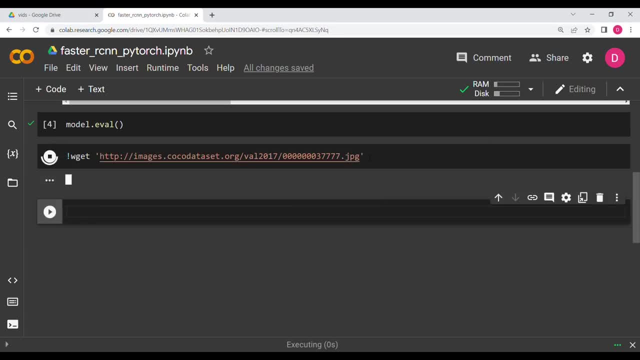 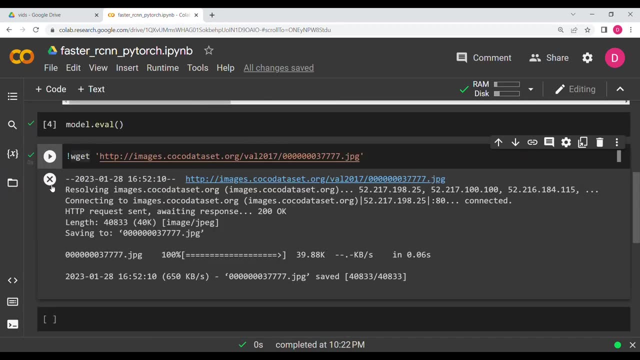 It's in the description, you can go and see. So this is the image, okay, And you can see over here. You can see the image has been downloaded. Now what we are going to do, we are going to read this image. So let's say ig, it's a variable. We will say image dot open. 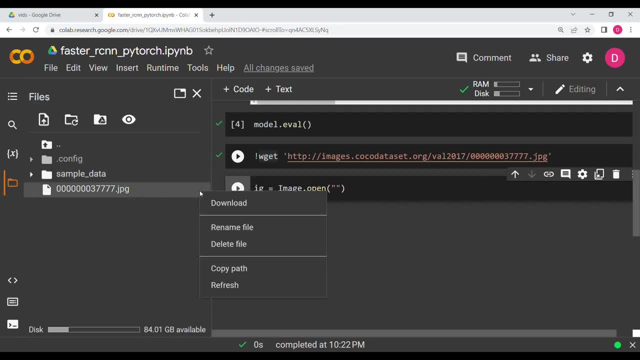 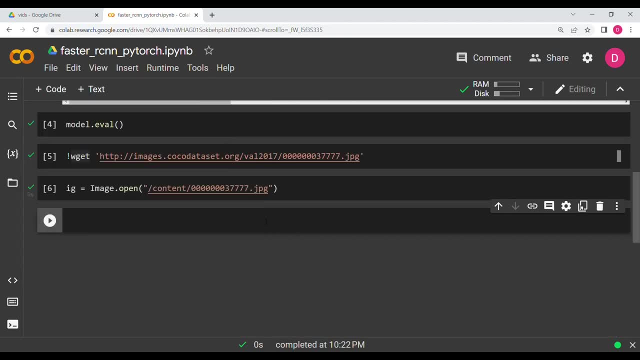 And then we are going to pass the path. So here we will go and we will copy the path, So this will open The image using the pil library. okay, Now what we are going to do is we are going to say, um, transform. So again, this is transform without the s, and the package imported is transforms. Okay, so there is a difference. 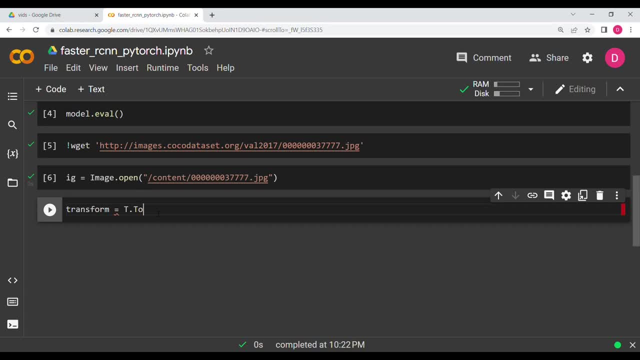 So we will say: transform equal to capital, t dot 2 tensor, And what this will basically do is it will help us convert the image that we have got from pil library to the Tensor format which will be given to the pytorch model. So for that i'm going to say image, which is another variable, img. 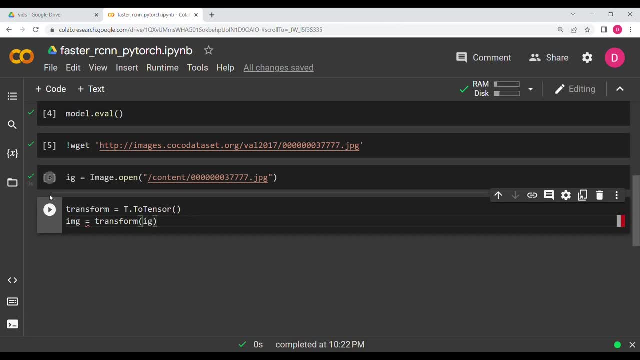 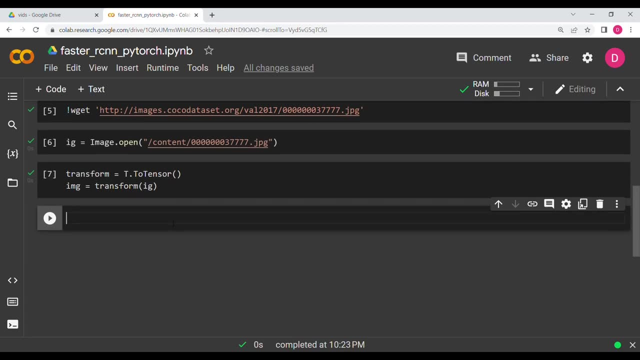 Transform and then pass in ig, which is the image that we have got in here, and then i'm going to hit shift and enter: Okay, Now what I need to do is I need to pass it, Pass this image to the model, but before that I need to say which: with torch dot: no grad. 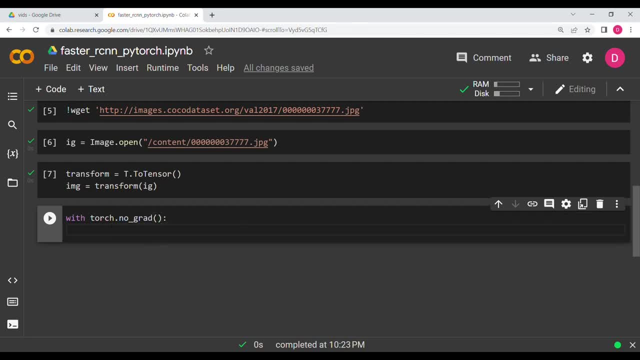 It basically means that we will not be using the grad gradient function Of pi torch and gradients won't be calculated. So this is there. and then, finally, we are going to say pred, equal to model, And with square brackets, i'm going to pass the img and i'm going to hit shift and enter. 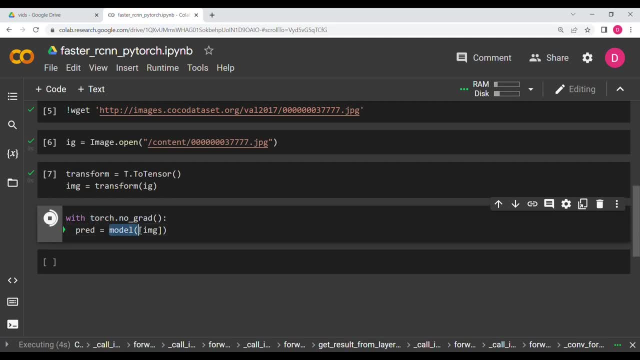 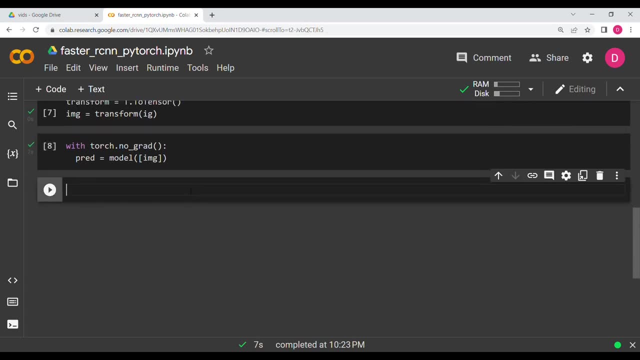 so this is expected to give the predictions, because In the model we have provided the image. Okay, so it takes some time. Yes, It has finished. So now what i'm going to do is i'm going to see what pred has given us. Okay, 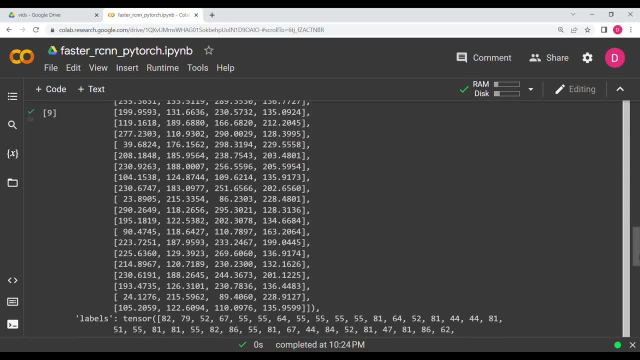 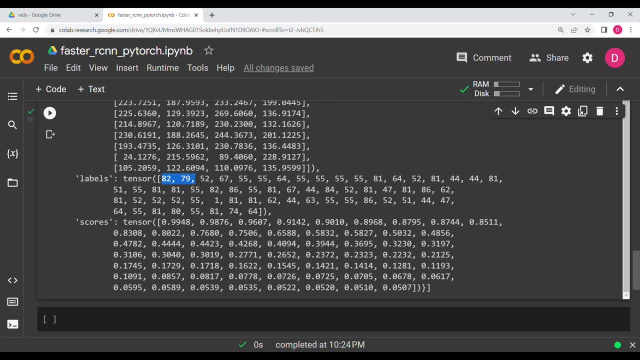 So i'll write pred and you can see there are a lot of values. So if you scroll down, you're going to see two things. two things: One is labels: This is basically the number of, or rather the objects that have been detected. And this is scores. Okay, so you can see the confidence. 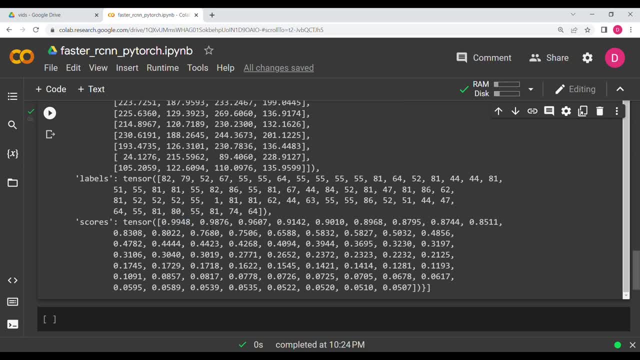 So for the first object It's almost 99.5 percent Sure. second object is 98.76, then third object is 0.9607, and the other things. interesting thing is here that all these numbers are in descending order. okay. so the first object, whatever- is the 82nd. 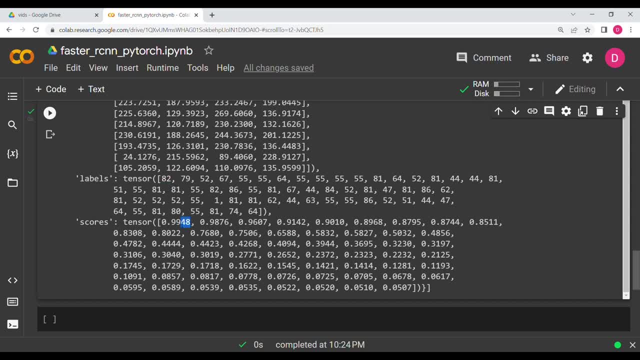 object. i'll show you, i'll be giving you the labels in a second to see what actually is that. so 82nd object has a probability of almost 99.48 percent, or yeah, 99.48 percent, or rather almost 99.5 percent. 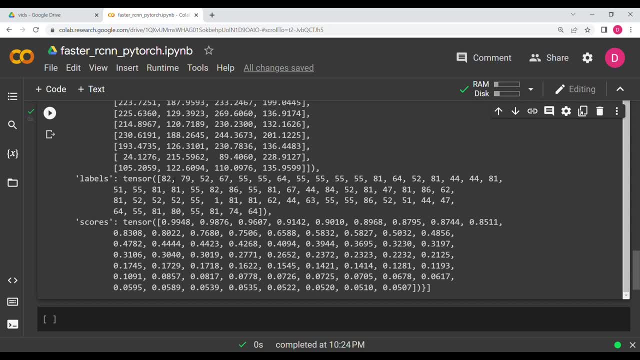 the model. is sure that the object 82 is there. now, what is object 82? i'll give you in a second. then, for object 79 over here, it is 98.76, sure. for object 52, it is 96.07, and so on and so forth. okay. 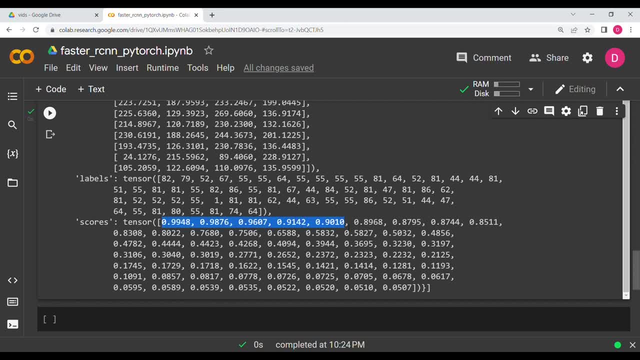 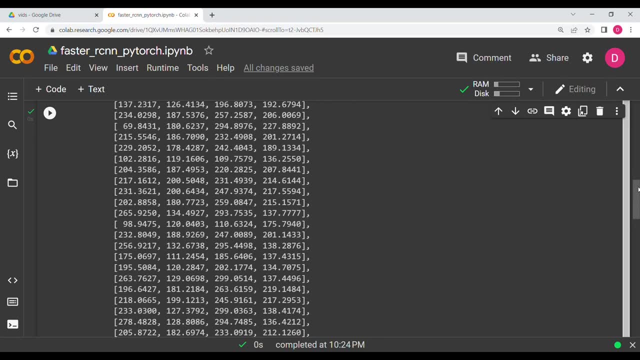 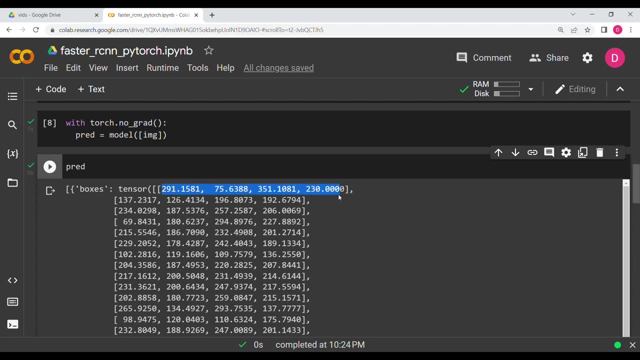 so, as you can see, there's so many objects that have got 90 and above. so i think the model is pretty sure, and the top one that over here you can see, these are actually the bounding boxes, okay, so, so, so, so you can see, over here the first row has four elements, okay, so this is the first element. 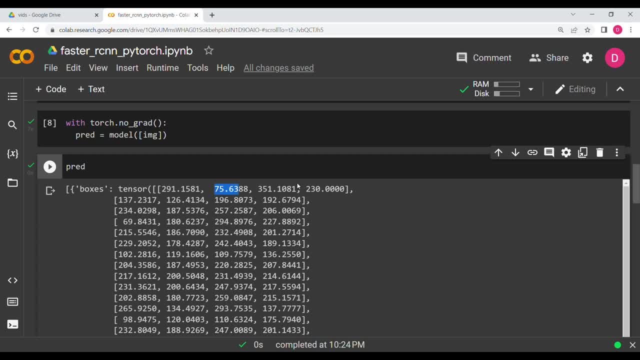 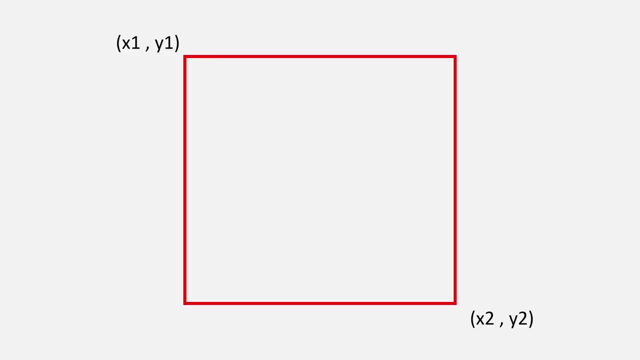 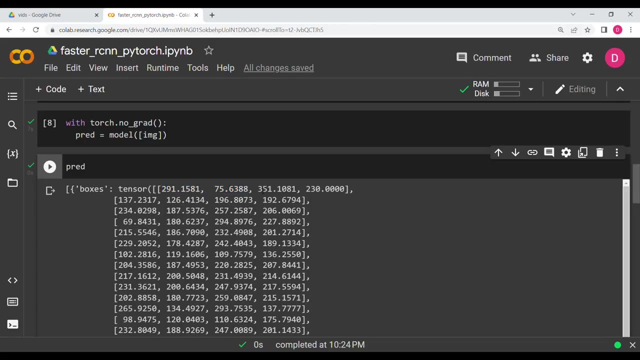 oh sorry, this is the first element, this is the second element, this is the third element and this is the fourth element. so these are the x1, y1, x2, y2. as you can see in the image, this one x1 and y1. this is the top left coordinate, as you can see in the image right now and this one over here. 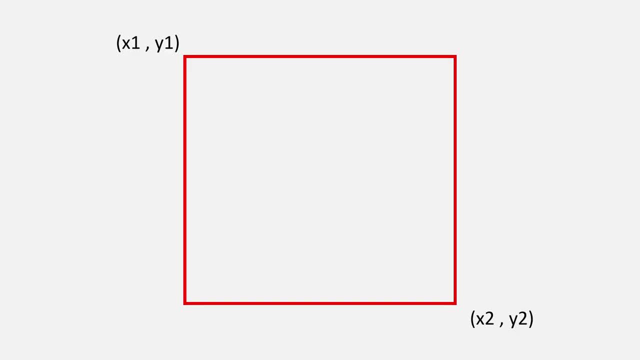 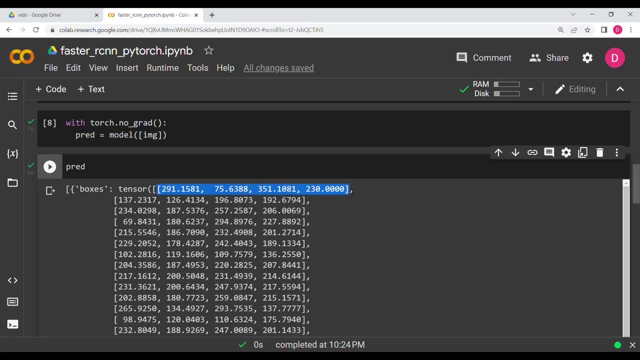 this, these two, this is x2 and y2. this is the bottom right coordinate which you can see in the image. okay, so for every bounding box, there is a x1, x2 and y1, y2, or rather x1, y1 and x2, y2. 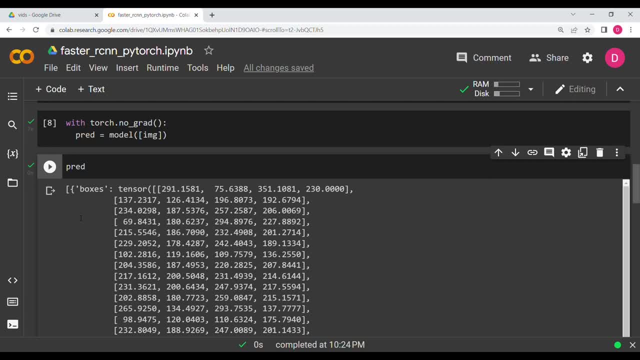 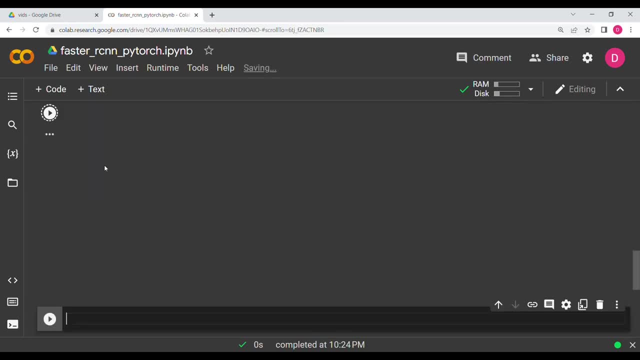 so this will help us making the bounding box. so what i'm going to do right now is: you can see there are three of them. if i'm going to show you, i'm going to show you here, i'm going to write type, okay, so if you see, um, give me a second. yes, 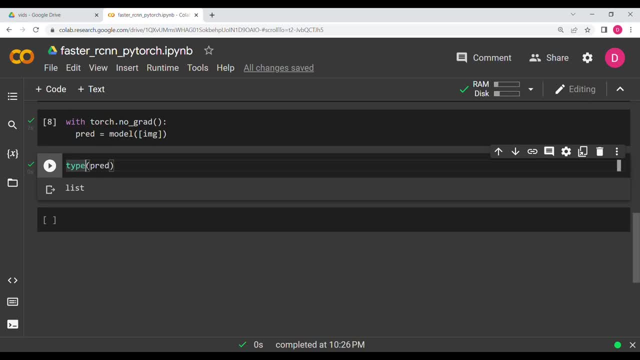 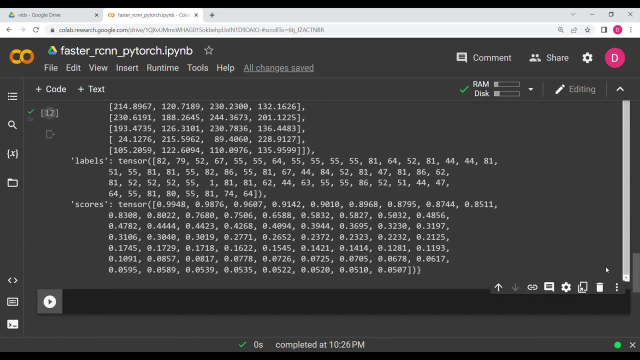 so you can see the type of pred is list. so if you see the length, length it will come one. so if, if it has only one element, then i'm going to say pred of zero. okay, so if you say pred of zero, you can see there are those elements. what those outputs that we saw? 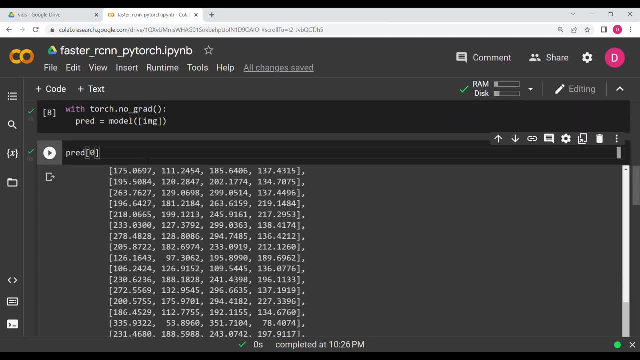 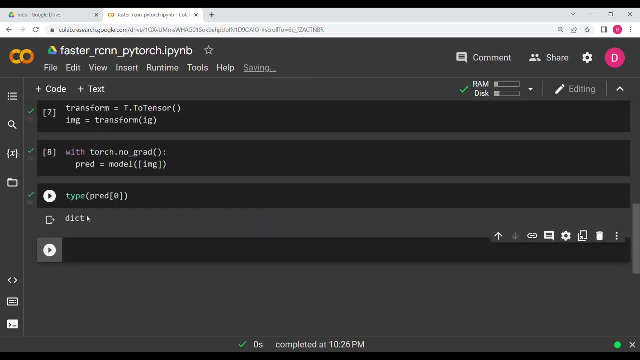 it's here. now let's see what these elements are. okay, the types, or the, rather the type. so i'm going to say type pred and you can see this is a. you can see over here. this is a dictionary, okay, so. So if this is a dictionary, then we obviously are going to have the keys. So if I write dot keys, 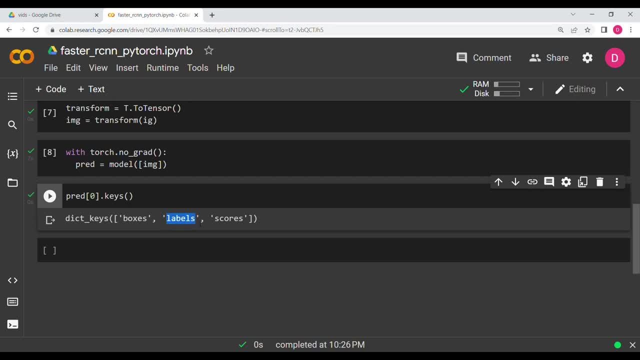 I am getting three keys. Obviously, we saw the bounding boxes, we saw the labels and we saw the scores. So what I am going to do is I am going to say bboxes, comma labels, comma scores, and now we are going to separate this into different variables. So for that, we are going to say: 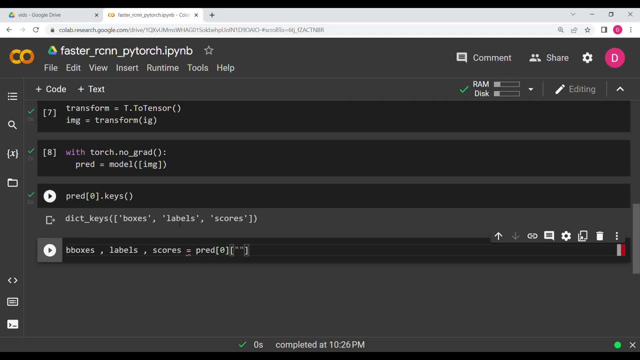 pred of zero, and since it was a dictionary which has a label- boxes, you can see, is boxes- I will copy it from here directly and then paste it over here. Then what I am going to do, I am going to copy this entire thing and then paste it twice and here, instead of boxes, we will have labels. 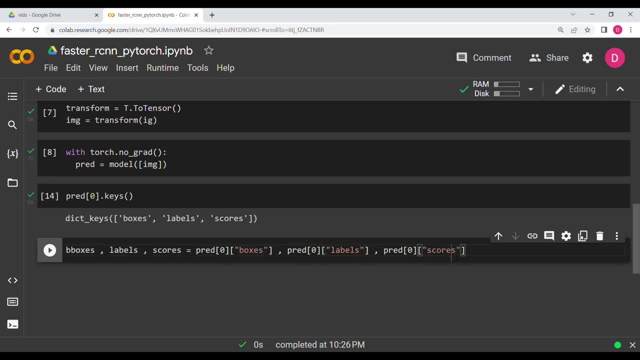 Labels, and here, instead of boxes, we are going to have scores. So whatever the scores that we had seen over there will now will be stored in scores variable. The labels here will be stored in the labels variable, And so for the boxes, Then we are going to hit shift and enter, and this has run. 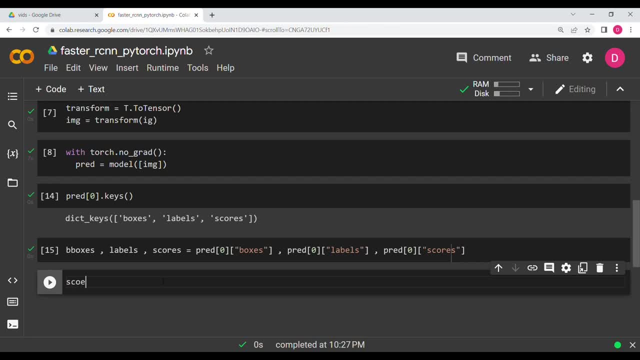 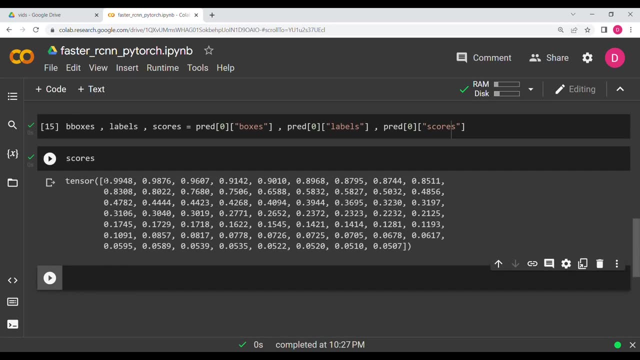 So now what we are going to do is: let's take a look back at scores. So if you look at the scores, what you are going to see is that there are certain scores which are in descending order, which I have already explained, but there are many, many objects, So I only want to see the top five. 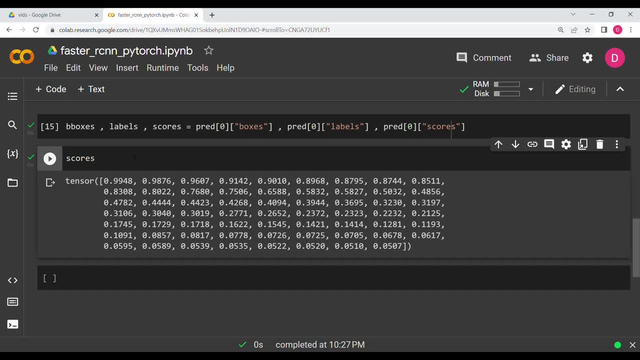 So I don't want a lot. So what I am going to do? if I have a condition- let's say that scores have to be greater than 0.9- then only the top five will be taken. Right, Only the top five will be taken. 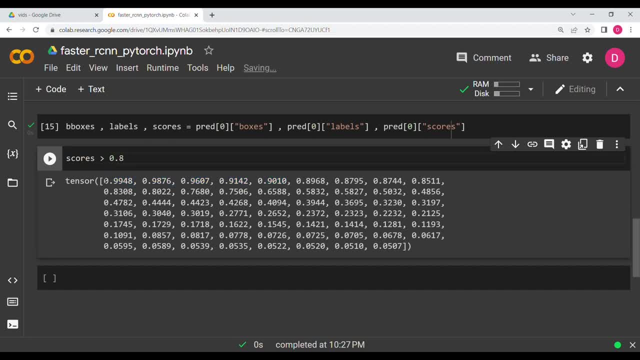 If I say 0.8, then till here it will be taken, because still here, till this last one, the probability is greater than 80 percent. So let's just keep it to nine. And the way to get how many objects will be be there, well, there will be five objects. so to get it in form of a number, i'm going to say torch. 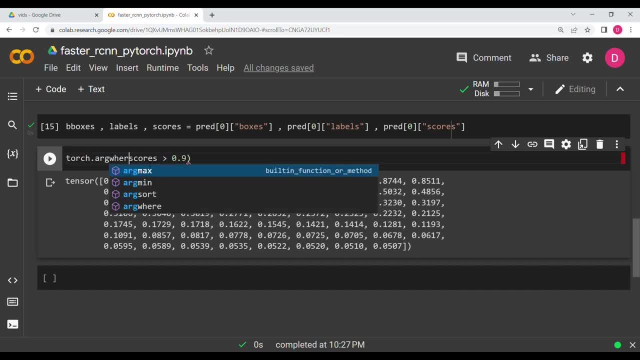 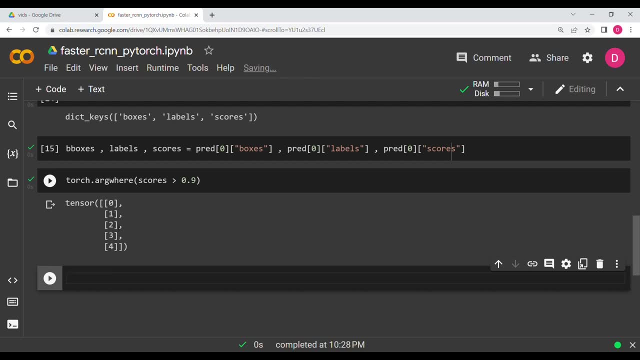 dot, arg, dot, arg, where. and then pass this condition and if i hit shift, enter, you can see there are five numbers: 0, 1, 2, 3, 4, 5, which means at position 0, at position 1, at position 2, at position 3 and 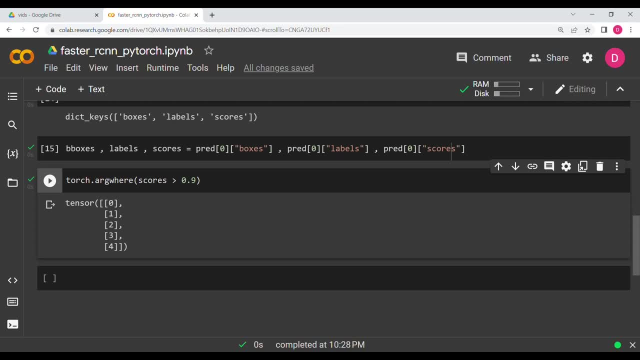 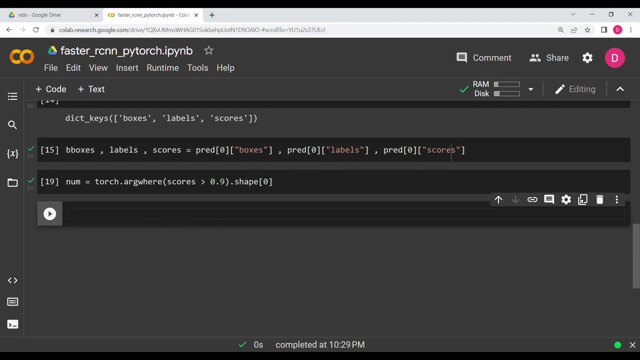 at position 4, all these five positions, the score was greater than 0.9. now, if you get the shape of it, you will actually get the number, which should come five. so you can see five. now i'm going to save it as a num, and now what i'm going to do is i'm going to give you the names so you don't have 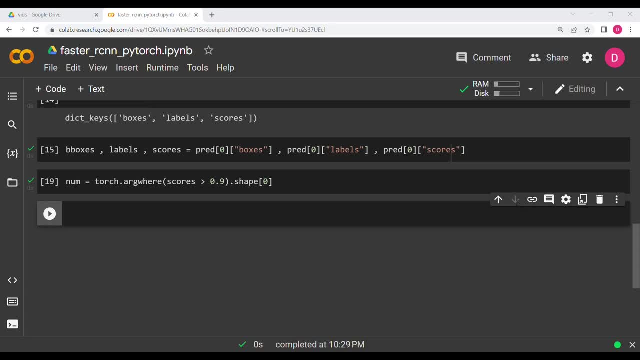 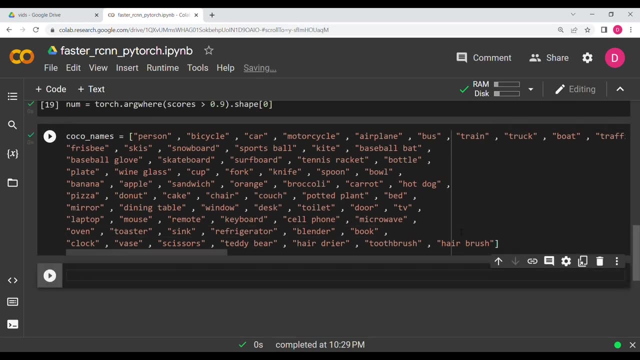 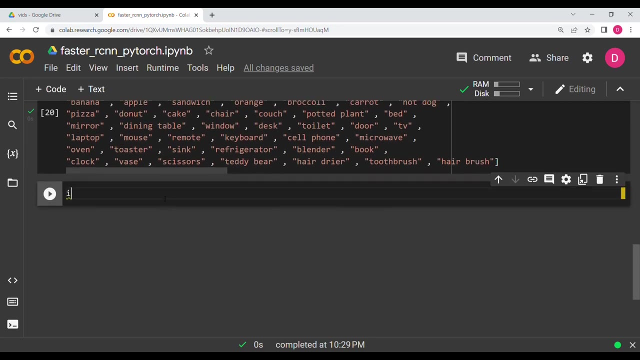 to worry, it's already there in the uh description. you can directly go and copy. so i'll copy from there and paste it over here. so these are the name of all the classes that we will be using to get the labels. okay, now, what i'm going to do is i'm going to write the um, what to say? your? 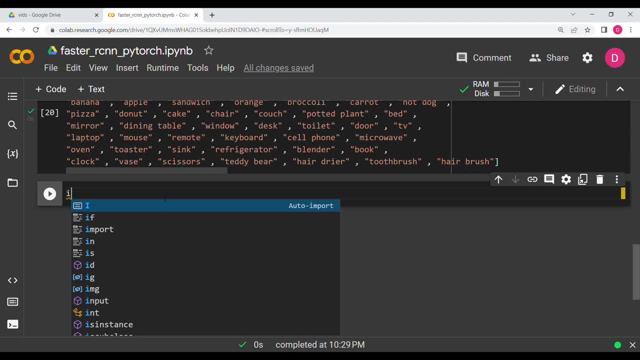 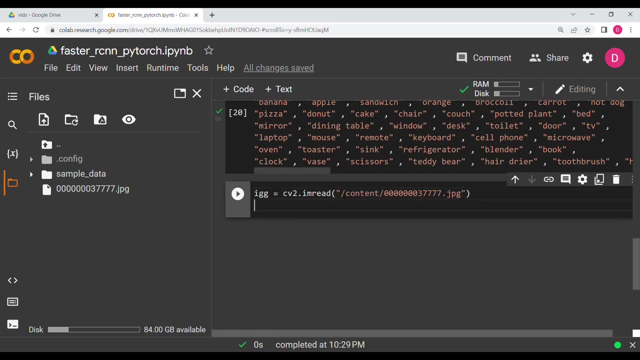 loop and finally make the prediction and show you the image. so i'm going to say igg, which is a variable, and i'm going to read the image in cv. okay, so now what i need to do is i need to copy the path. i'll again go there and copy the path. okay now, how many objects we have to display? it is there in. 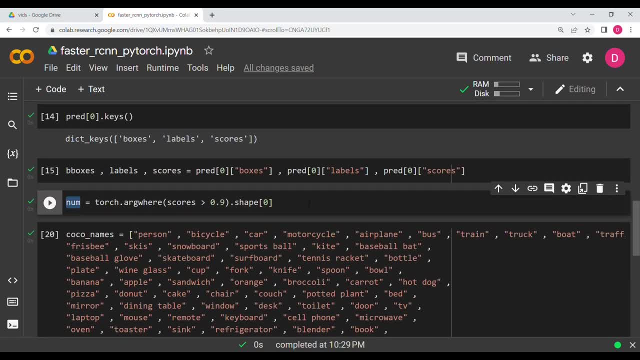 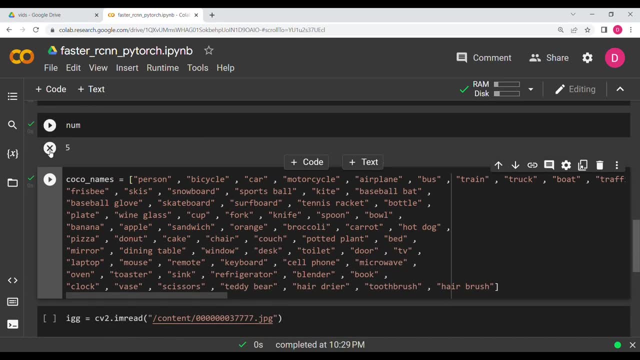 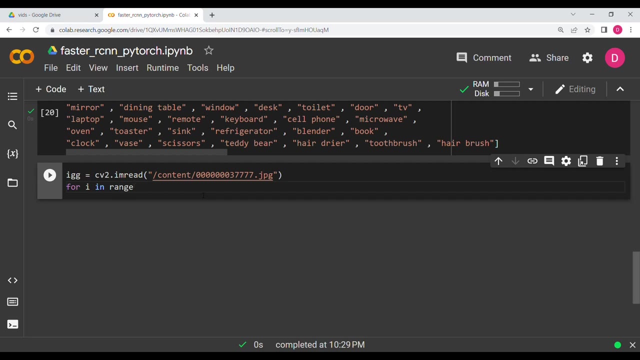 the value num. if you remember, num is five. okay, i can also print it over here: num is, num is five. as you can see, num is five. fine, now coming back. so i'm going to say for i, in range of a num now, for every uh range, what i'm, every uh number in i, what i'm going to do, if you remember from, 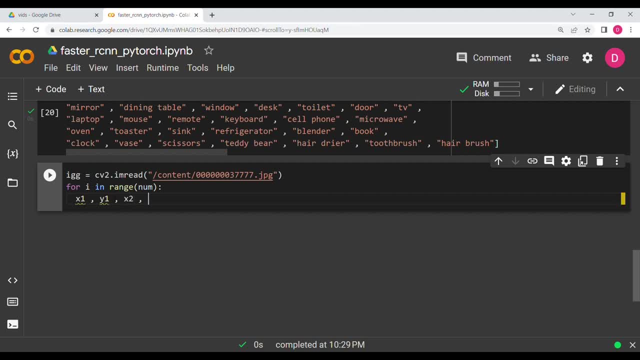 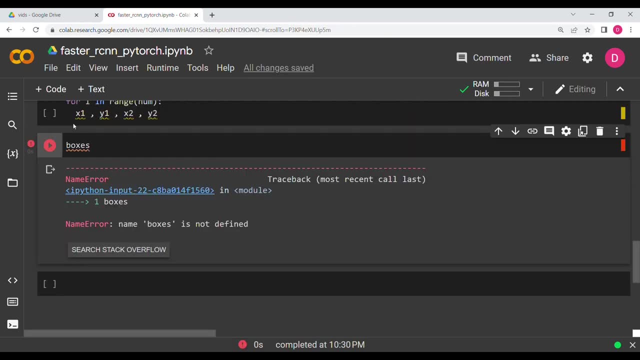 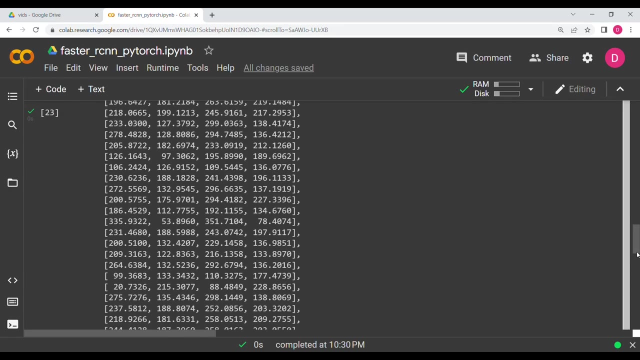 the boxes. i'm going to write x1, y1, x2, y2 and, for your reference, i'm going to actually print the boxes over here so that you can see: oh, not boxes, b boxes. my bad, so, um, I'm going to write, sorry, I'm going to write B boxes. Okay, So, as you can see over here, 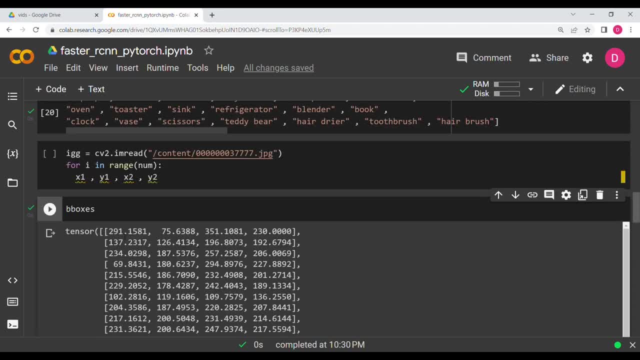 these are our bounding boxes. and see, there are four values in every row, So X1, Y1, X2, Y2.. And what I'm going to say? I'm going to say B boxes. I Okay The other thing you can see here. 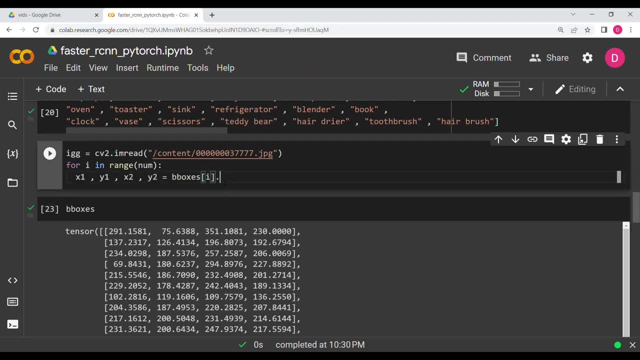 is. this is in tensor format and I want to use it in numpy format because I'll not be able to print it. print it otherwise. And the other thing is there, as you can see, this: that this here is in decimals but coordinates, you know, has to be in integers. So for doing that, I'm going to write. 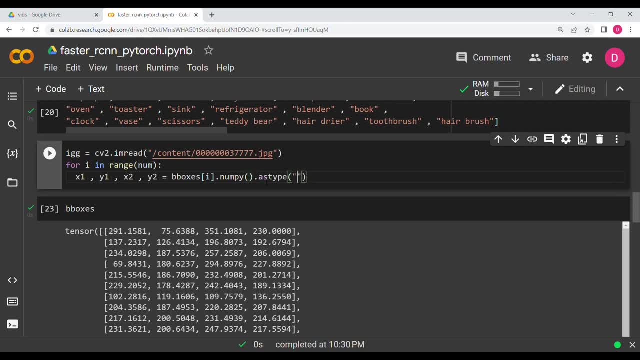 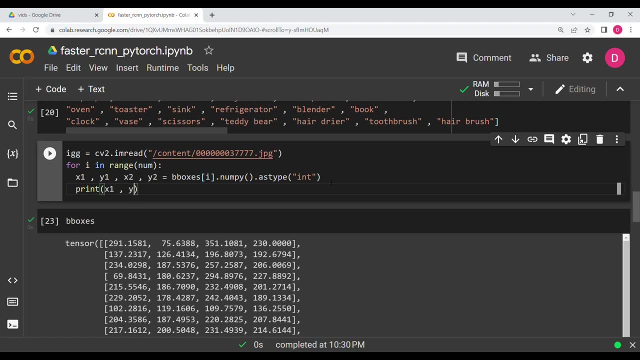 dot as type, and then I'm going to write int: Okay. So now what you're going to see is if I run this and let me, just for a second, print X1, Y1, X2, Y2.. And then, finally, I'll break. Um, finally. 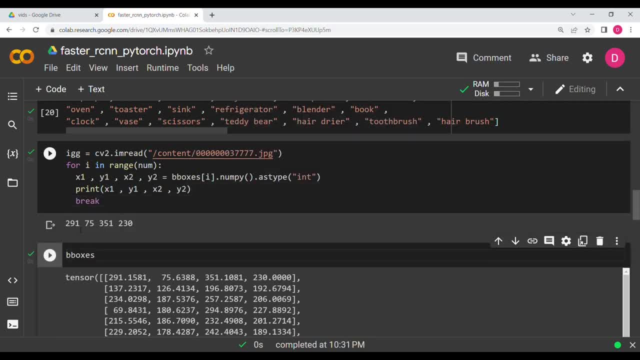 after that, I'll just break in order to show you. you can see 291.. You can see over here, 291,. you can see 75,. you can see 75,. you can see 351,. you can see 351,, 230,, 230.. So it has gotten the integer parts of. 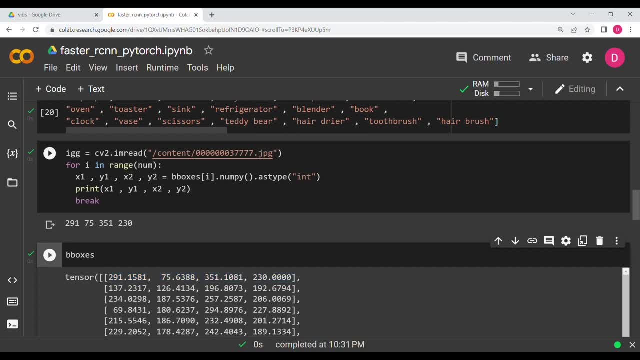 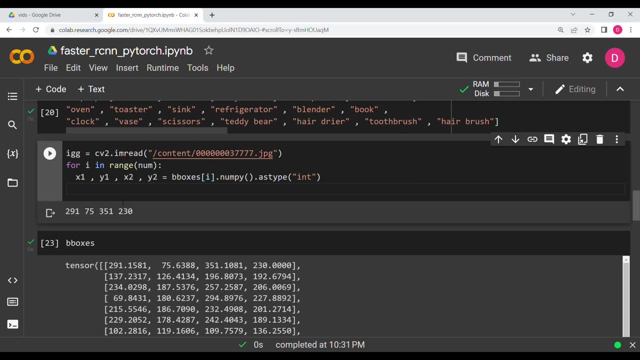 the first row, And so the next time, when I will be equal to one, it will get the second row, and so on and so forth. Okay, So now what I'm going to do is I'm going to say: um, class name, class name. 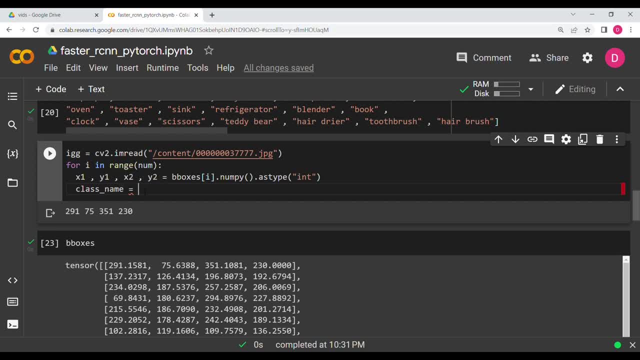 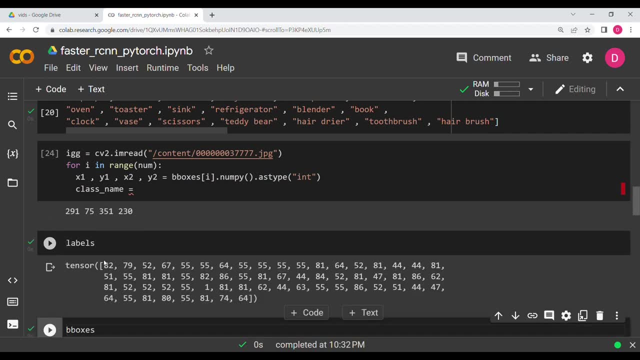 is equals to now what is class? Basically, this is going to get us the labels. For example, if you print the labels, I'm going to print it for you. So the thing is that, see, you can see 82 over here. Now the problem is how to. 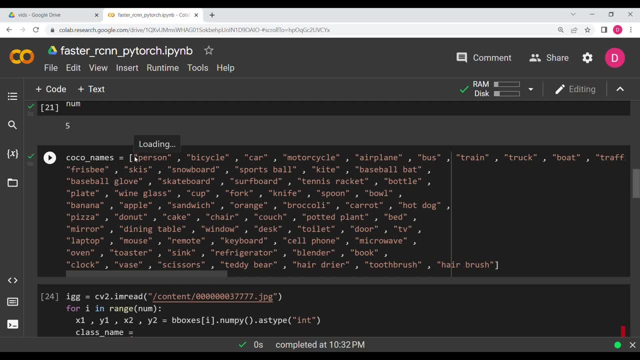 know that which label it corresponds to, It corresponds to the 82th level. So the person is one, bicycle is two, you know, car is three, motorcycle is four, and counting that, wherever it comes to 82, that is going to be our label. Okay, So what I'm going to say. 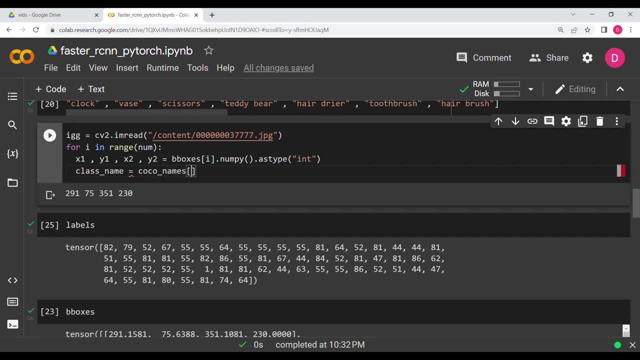 I'm going to say Coco, Coco names, And since label is there, so we are going to say labels dot numPy, because it's also in tensor format, as you can see over here, And then I'm going to say I minus, or I minus one, Y minus one outside, Because, remember, this is a list, Okay, This Coco. 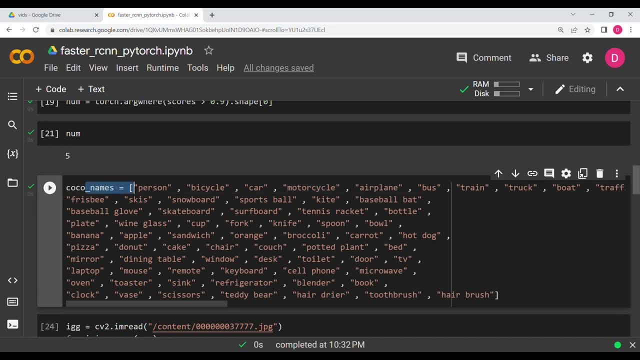 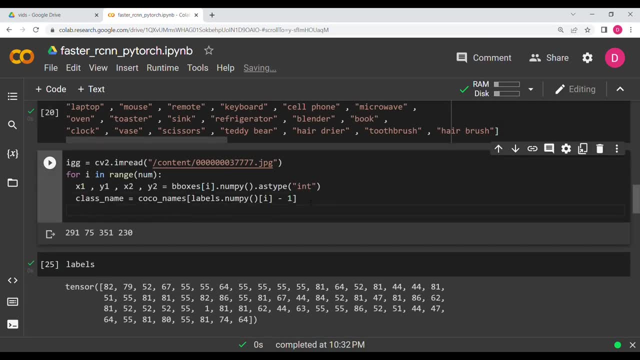 names over here. as you can see, this is a list. list is index, not from one, but from zero. That's how we have to subtract minus one here. okay, so with that we'll get the class name. now what i need to do? i need to print it, so i'll. 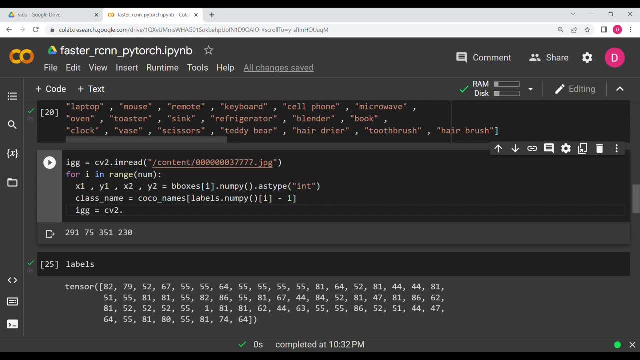 say igg, i'll, i'll print the bounding box. okay, so first i'll print the bounding box. i'll say cv2.rectangle and rectangle. for that i have to give the image igg, the top left coordinate, if you know it was x1 comma y1 and the bottom right coordinate is x2 comma y2. then i have to give the 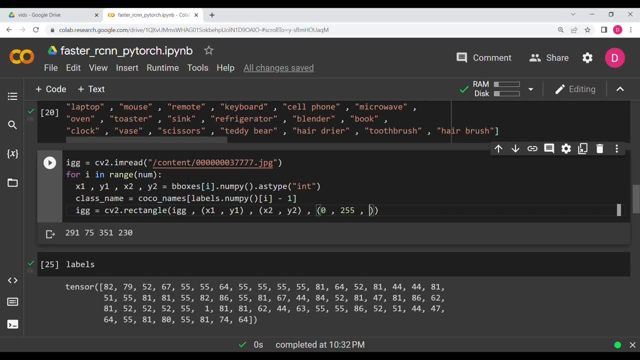 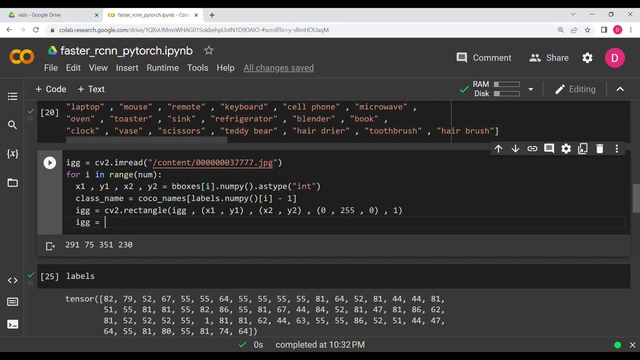 color. i'll be giving it green color. so 0 to 55 and 0, and then finally, i'll give the thickness as 1. lastly, i also want to print the class names, so again, i'm going to use the cv2.put text function. 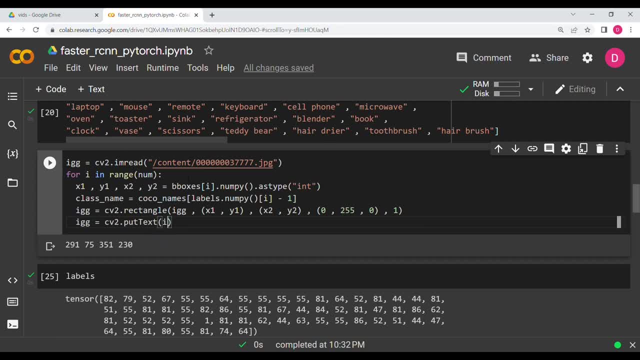 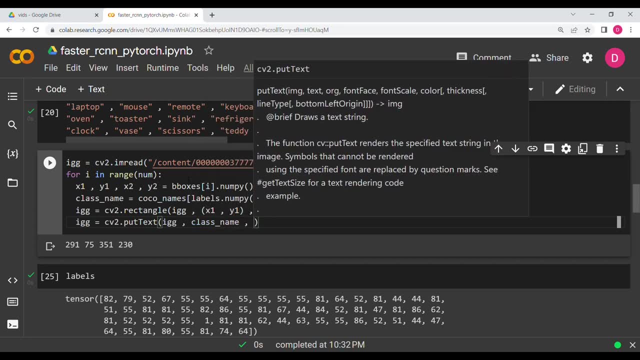 okay, and for that i need to give the image, then i need to give the class name. i'm going to say class name only- and then i need to give the coordinate which i'm going to give it. so where do we want? we want it on top of the box, so we need to take the. 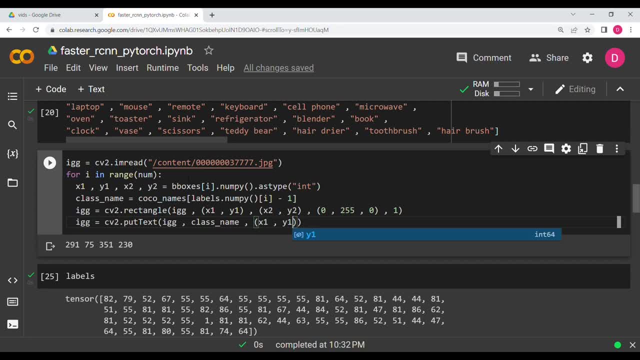 top left coordinate, which is x1, y1, but i want it at the top, so i'm going to reduce 10 from the y1. i hope you are familiar with the coordinate system for images when it comes to opencd. okay, so after that i need to pass the font. so i haven't mentioned the font here, so i have to. 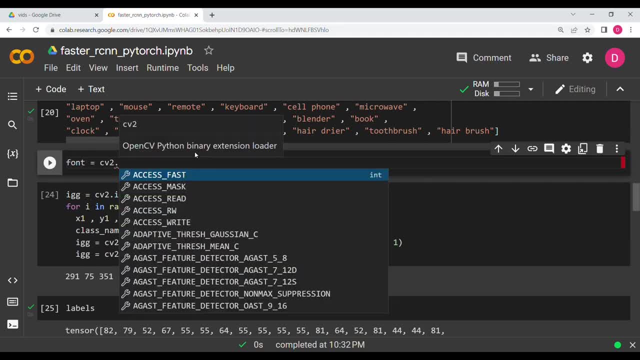 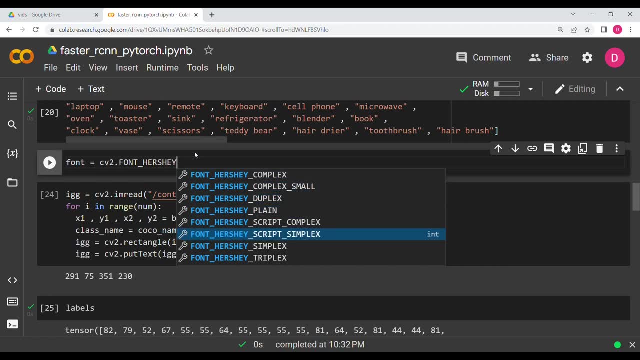 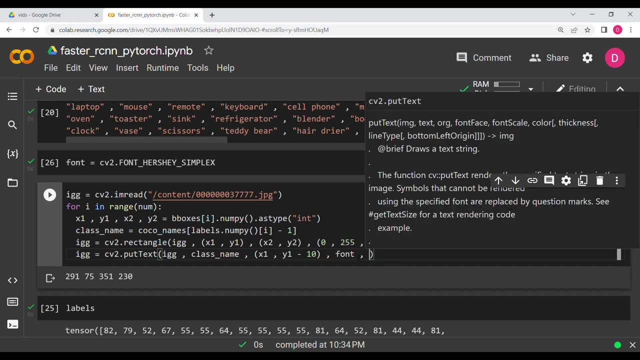 say: font equal to cv2.cv2.font. hershey, hershey, simplex. i'm going to just simplex. okay, so this is the font i'm going to use for the image here. so i'm going to say font equal to cv2.cv2.font- our font. now, after that, what we need is we need to give the um, let's say the thickness. so, uh, no, 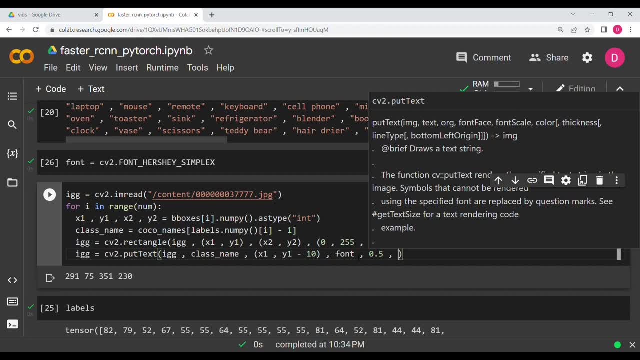 not the thickness, the font size, so i'm going to keep it 0.5. i don't want the font to be very, very big. then i need to give the color, so here i'm going to give blue. so 255 comma 0 comma 0. okay. 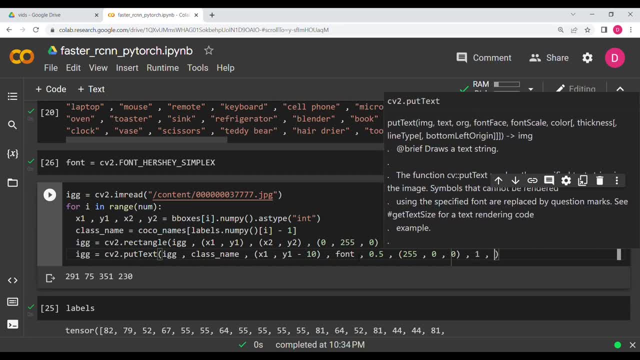 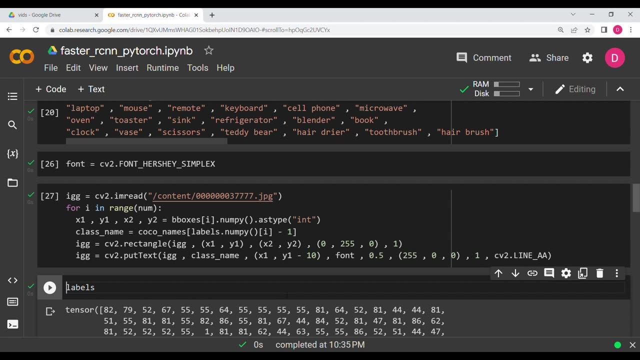 after that i need to give the thickness, so i'll keep it as one. and then, finally, i have to write cv2 dot line under cv2, cv2 dot line underscore aa. okay, so i'm going to hit shift and enter and this has run. now what i'm going to do? i'm going to show you the image, so i'm going to say: 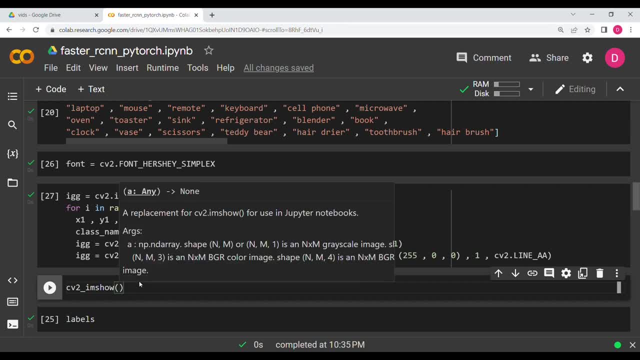 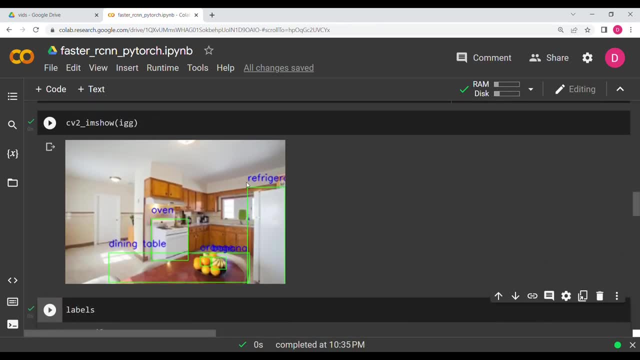 cv2 imshow and i'm going to show you the image. so i'll say: igg, so let's see what we get. so, as you can see, we have got an output. uh, refrigerator is here. refrigerator is here. you cannot see it over here, but i know it is a refrigerator and you can see it in the image. 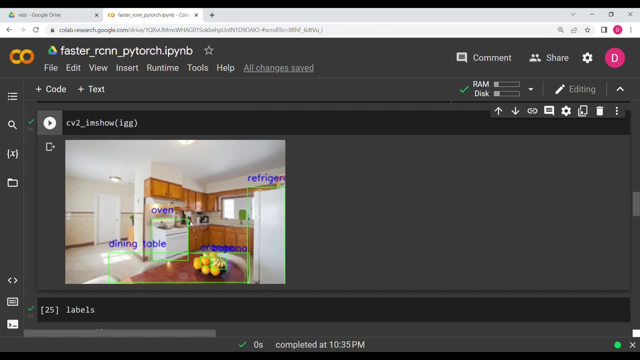 also that it has detected the refrigerator. you can obviously see the oven here, so it has clearly detected the oven. it has also detected the table. as you can see over here the dining table is written, and it has also detected an orange and some bananas. so obviously this is occluded, but 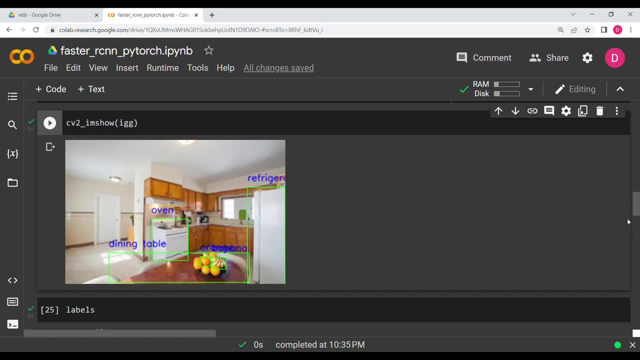 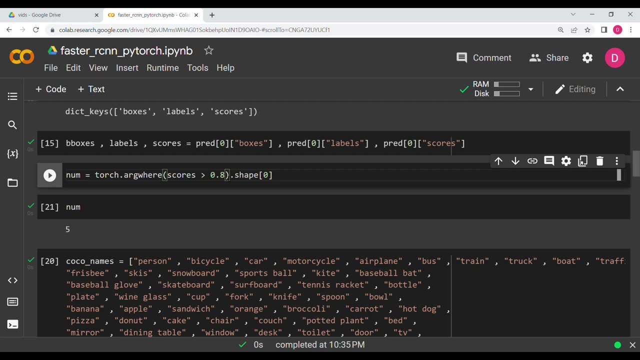 you can see in the image that there are certain objects that have been detected. now, remember we have kept the confidence very, very high: 0.9. if i reduce it to 0.8- okay, then you'll have more objects. so you'll see the number has changed, okay, and num will change. it will come to 11 because now 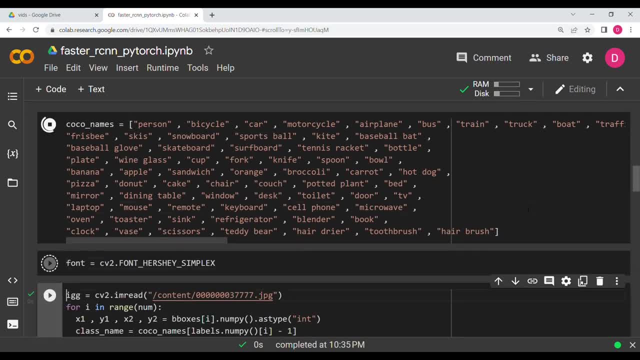 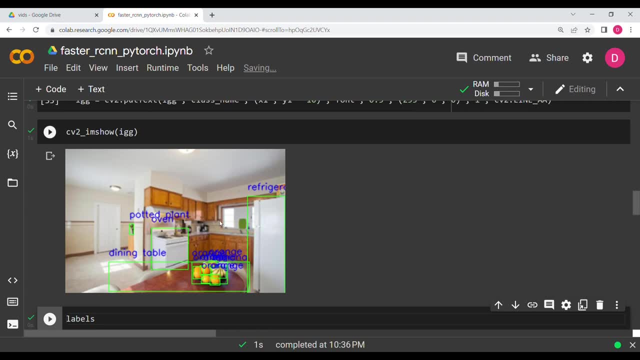 we have given more objects, so this will remain the same. this will remain the same, and in here i'm going to let's see what we get over here. so, as you can see, some more things have been spotted. so, for example, potted plant- okay, this has been spotted. a lot more oranges have been. 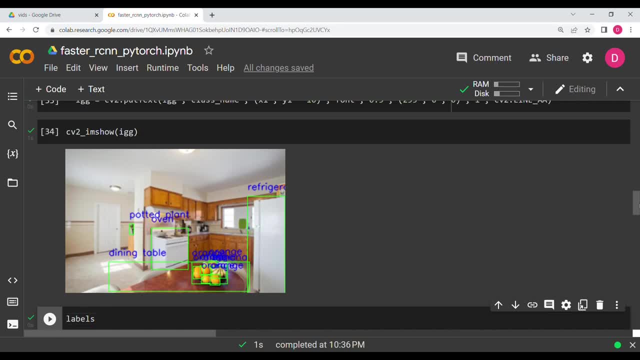 spotted. so, for example, potted plant- okay, this has been spotted. a lot more oranges have been spotted. so, for example, potted plant- okay, this has been spotted. a lot more oranges have been spotted and the bananas itself. so you can see the object detection kind of works and 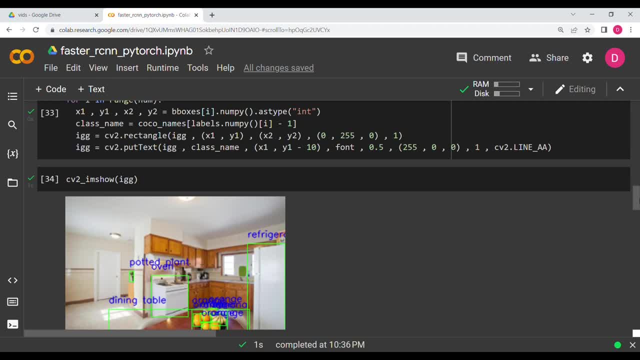 it gives us good enough results, okay, so I hope you understood the video and the code and everything will be there in the description. thank you and bye.